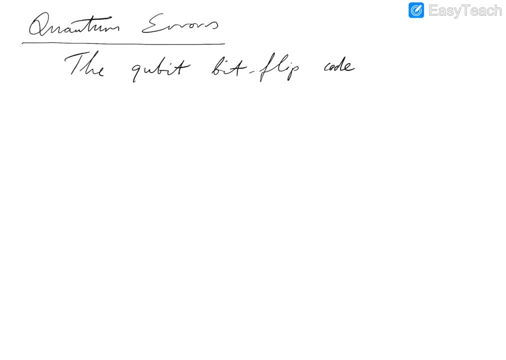 So suppose that Alice wants to send some quantum information through some faulty communication channel to Bob. So suppose that Alice wants to send some faulty communication channel to Bob And we assume that the faulty channel has the characteristic of the bit flip error, the bit flip model. 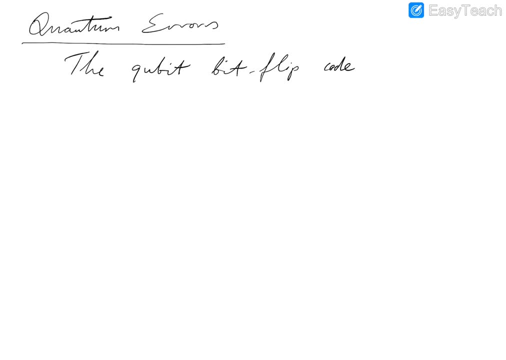 And the qubit gets flipped with probability p and it's left unchanged with probability, let's say 1 minus p. Okay, so now assume that Alice wants to send. so Alice, Alice wants to send qubit phi a0 plus b1 for some unknown values, a and b- through the bit flip noise channel. 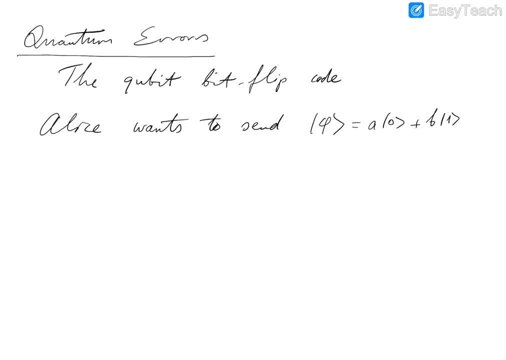 Okay, so now what we do here in this protocol is that Alice prepares two more qubits, Ancillary qubits. okay, Each set to state 0.. So we have the state that Alice wants to send, This is phi, And we have two more qubits. 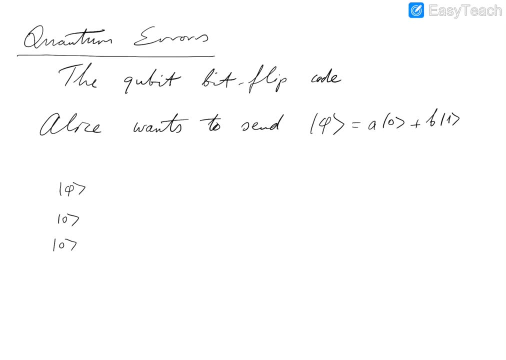 Ancillary qubits, So we have a three-qubit code. Okay, this is where the name comes from. And then Alice codes her single qubit state Into a compound state of three qubits and using two c-knot gates. 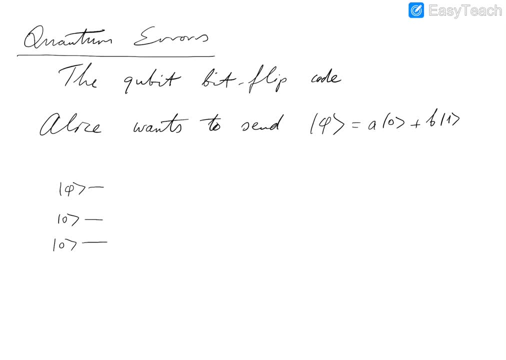 Okay, so she's going to use. this is the encoding procedure. she takes the first qubit as a target qubit, the control qubit. sorry, She takes the first qubit as the control qubit and applies the c-knot. 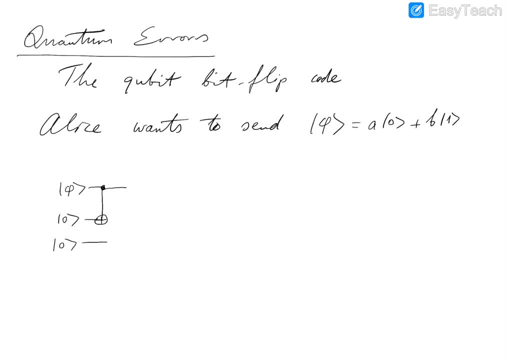 Transformation on the second qubit, And then she also takes the first qubit as the control qubit and applies the c-knot transformation on the third qubit. So this is the encoding stage. So our qubit phi is encoded into a three-qubit state. 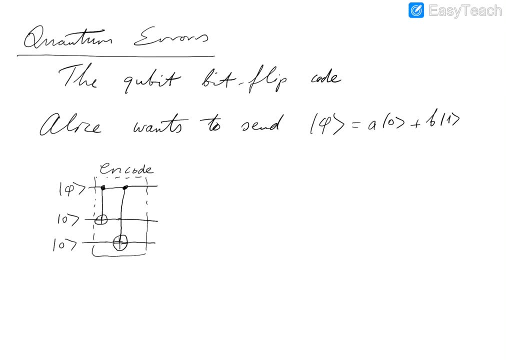 Okay, so then this encoded state, the three-qubit state, is introduced to the error model, The bit flip error. It's called ebit. Okay, Okay, and then, um, these three qubits are sent to Bob, And Bob, what he's going to do is that he's going to decode this compound three-qubit state. 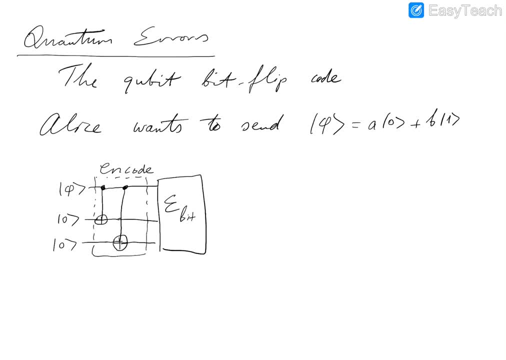 But he also likes to know what kind of which qubits were subject to the error. So he'd like to know the information about the error, That which qubits got corrupted during the trans, during the transmission. So for this he's going to prepare um. 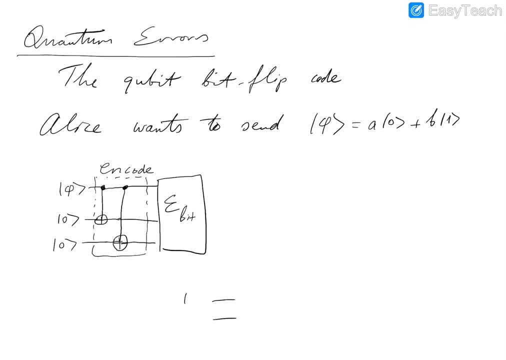 two auxiliary qubits set to zero initially, Okay. And then he's going to um take the first qubit as the control qubit And then he's going to apply a CNOT transformation on the first qubit of the ancillary qubit. 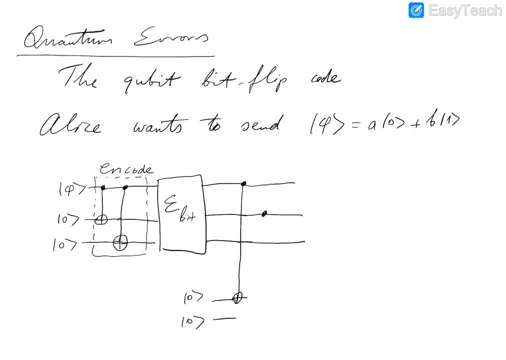 And then next he will take the second qubit. He's going to take this as the target qubit And then again he's going to apply another CNOT transformation And next he's going to take the first qubit as the control qubit. 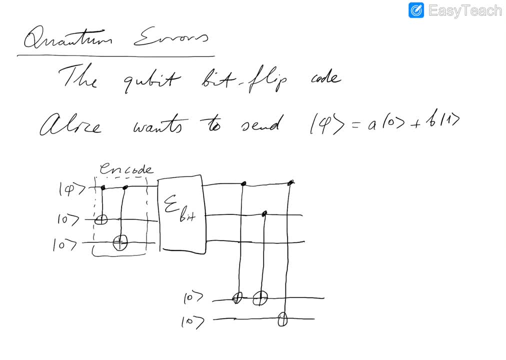 And then this goes to the second qubit. He's going to apply a CNOT transformation And finally he's going to take the third qubit here as the control qubit, And then this goes down to the second qubit of the ancillary state. 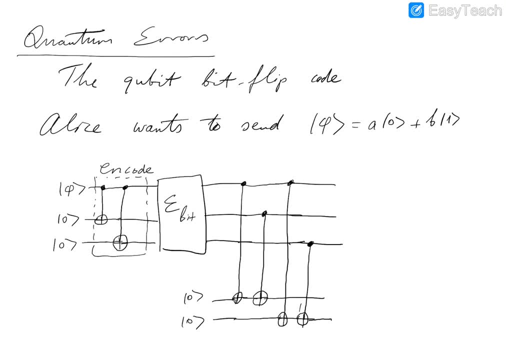 And then this goes down to the third qubit of the ancillary state. So this is the correction stage. So here actually this is called the last qubits. The last two qubits are called the error syndrome. The error syndrome gives us the information about the error occurred on the qubits. 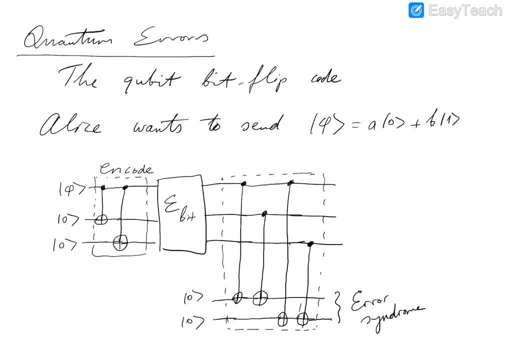 And then Bob will, respectively, accordingly apply a decoding operation in the receiving end. He will take the first qubit as the control qubit and apply a CNOT transformation on the third qubit. and apply a CNOT transformation on the third qubit. 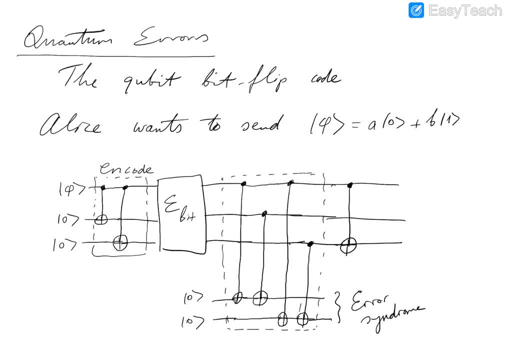 of the three qubit encoded states, And then next he's going to take the first qubit again and then apply a CNOT transformation on the second qubit and then apply a CNOT transformation on the second qubit. This last part is called the decoding stage. 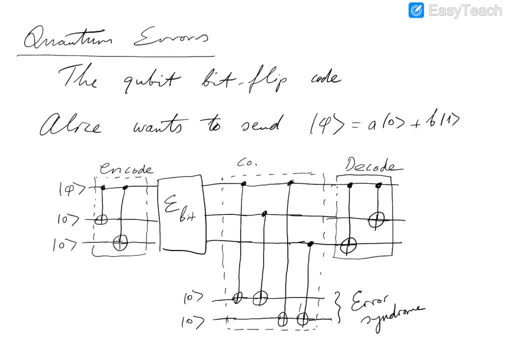 This is the correction. OK, so since we have the bit flip error model, then the correction will also be a bit flip transformation applied to one or none of the qubits, And this will leave Bob with a single qubit in state of phi. 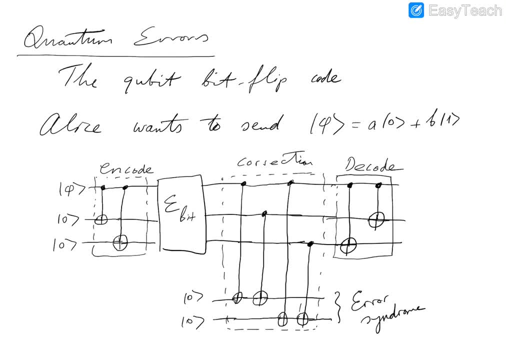 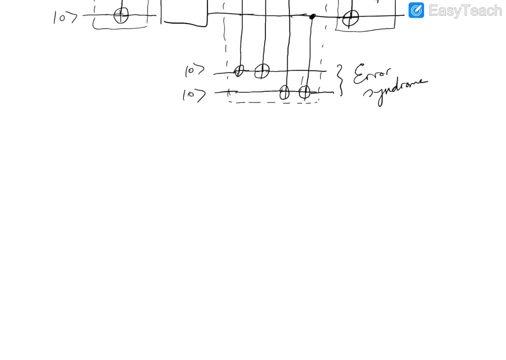 with probability one minus big O. with probability one minus big O. All right, so let's see how this works. All right, so Alice then wants to send. All right, so Alice then wants to send, Let's say, a zero plus b one. 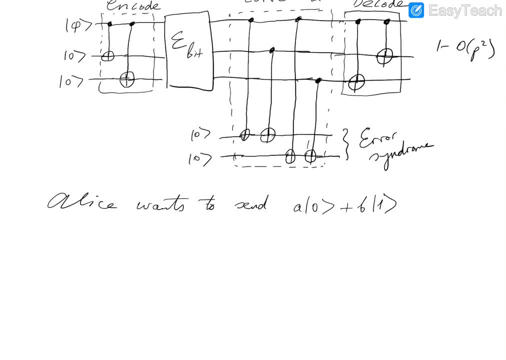 So then, with the additional qubit, So then with the additional qubit, With the additional qubits, the joint state, the joint 3-qubit state, becomes A0 plus B1.. And then we have the 2-qubit ancillary state 0, 0. 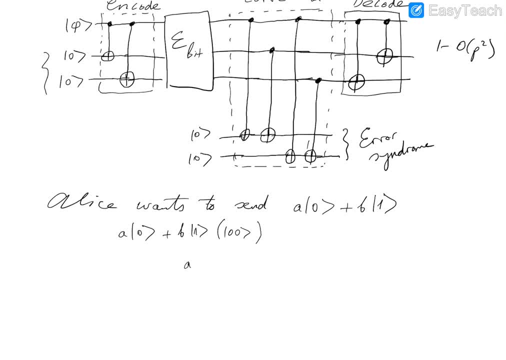 So this is equal to A0, 0, 0 plus B1, 0, 0.. So this is a compound state. Now Allison codes the state by applying a CNOT transformation. After the decoding stage we get: 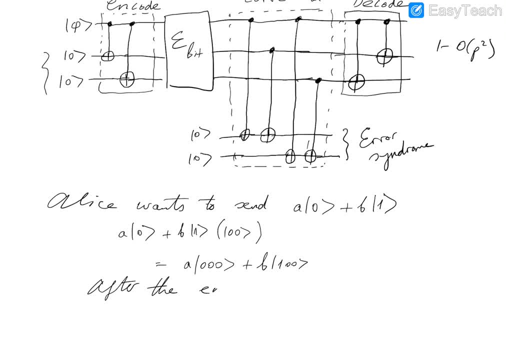 After the encoding stage. So the first part remains the same: A0, 0, 0.. And then we have B1, 1, 1.. So essentially, ket0 is encoded by the logical bit, The 3-qubit state 0, 0, 0. 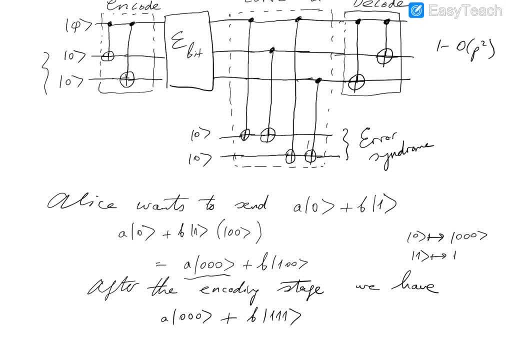 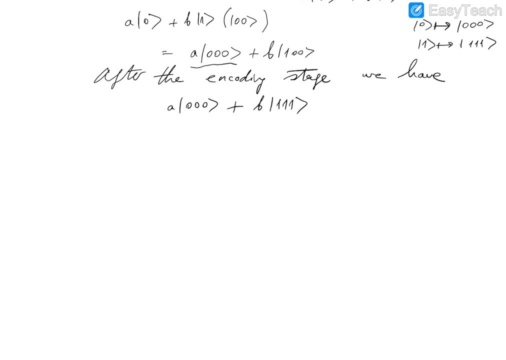 And ket1 is mapped to the encoded state 1,, 1,, 1.. Now Bob receives the 3-qubit state through a faulty channel or the noisy channel, And then He will receive The 3-qubit state either with no errors. 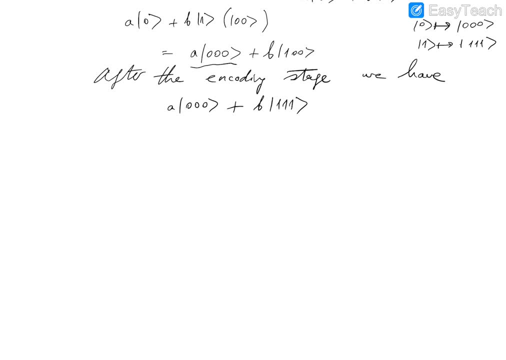 or a state where only one qubit is corrupted, or two qubits are corrupted, or maybe all qubits are corrupted, maybe. So let me draw a table to denote these. So if Bob receives a 0, 0, 0, plus B1, 1, 1.. 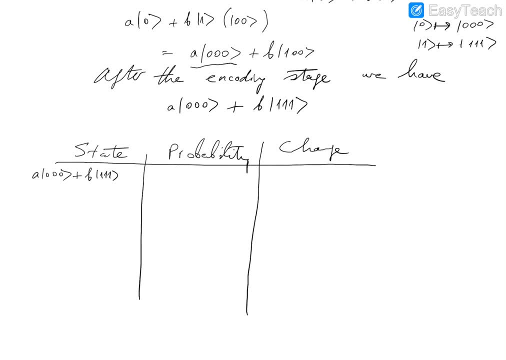 So we're talking about the first 3 qubits of the system. If Bob receives a 0, 0, 0, plus B1, 1, 1.. Well, the probability of Bob receiving this state is 1 minus p cubed right. 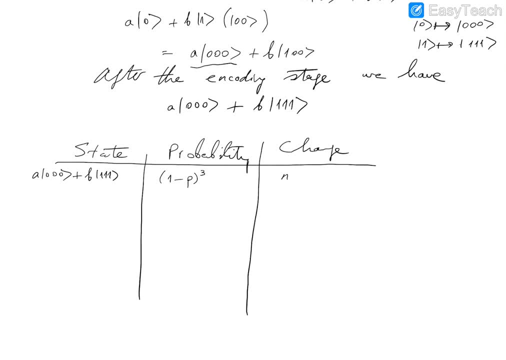 So in this case there is no error, so no change, Nothing's changed. This is exactly what Alice tried to send. If we have A1, 0, 0, plus B0, 1, 1 in the receiving end. 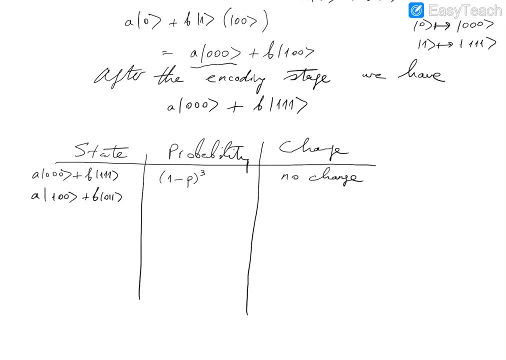 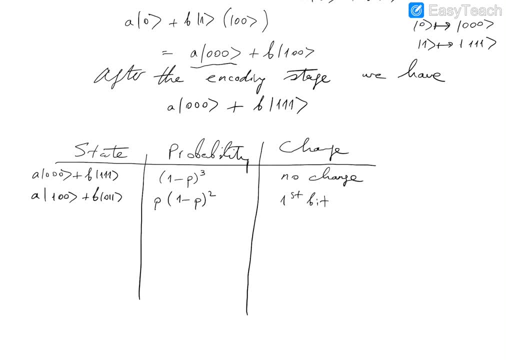 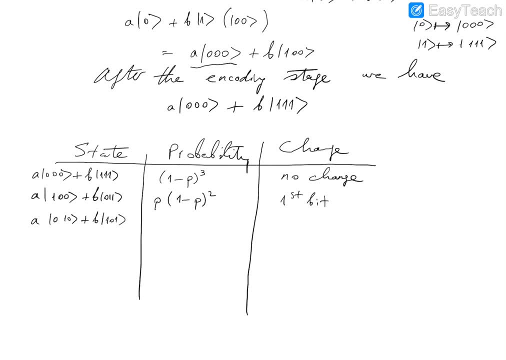 So yeah, in this case only the second qubit is changed And we have, So this occurs with probability the same as that, same as earlier: p times: 1 minus p squared. so only second qubit is changed here. second bit: if Bob receives a 0, 0, 1 plus B, 1, 1, 0, so that means only the. 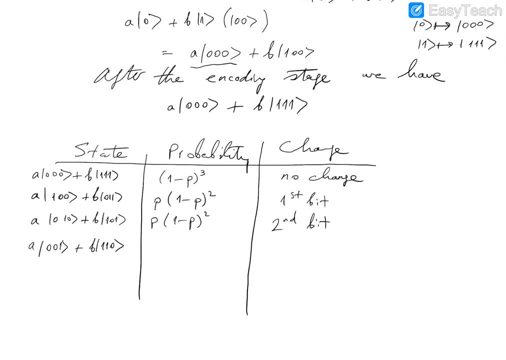 first qubit is changed. but it could also be that two qubits are changed. maybe the first and second bits are changed. so if Bob receives a 1, 1, 0 plus B, 0, 0, 1 and the Probability of this happening is p squared 1 minus p, so in this case only the first and 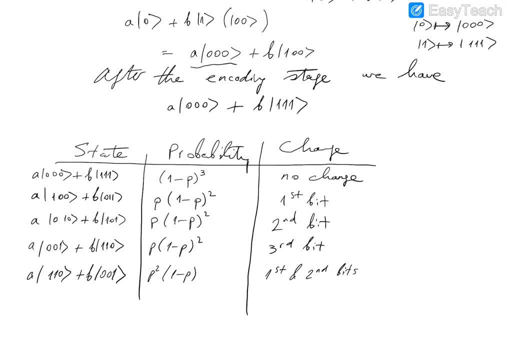 second bits. Another case would be that first and third bits are changed, so a 101 plus b 010.. The probability of this having this state is the same p squared times 1 minus p, And next, maybe second and third qubits might have changed: a 011 plus b 100.. 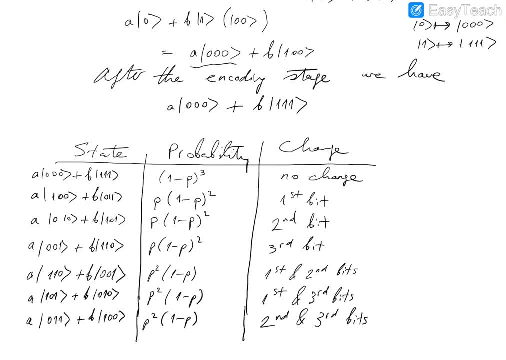 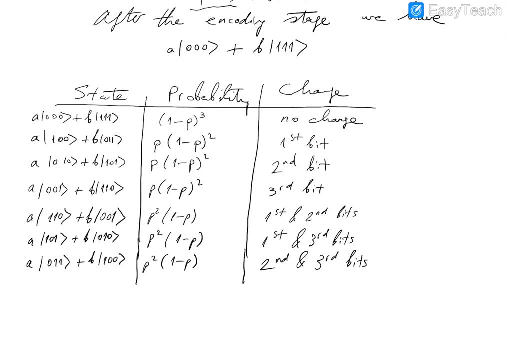 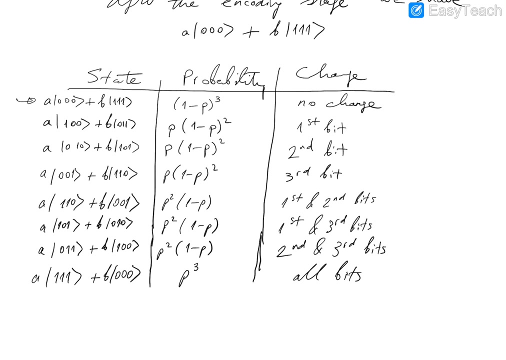 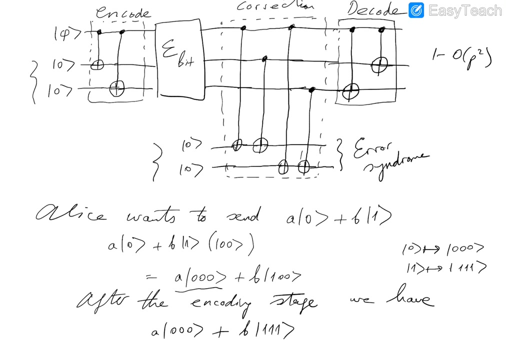 And then, finally, maybe all qubits are changed. So this entire state given here might have changed during the transmission, But the probability of this happening is p cube, all bits, All right. so now Bob prepares two more qubits and Scylla qubits, both set to zero. 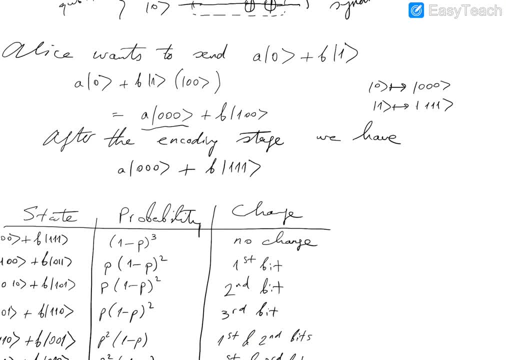 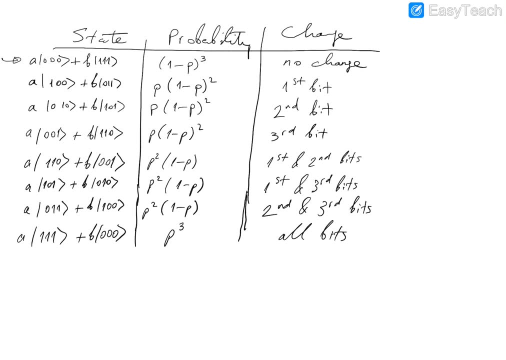 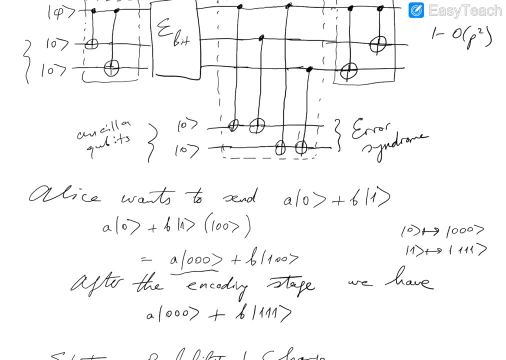 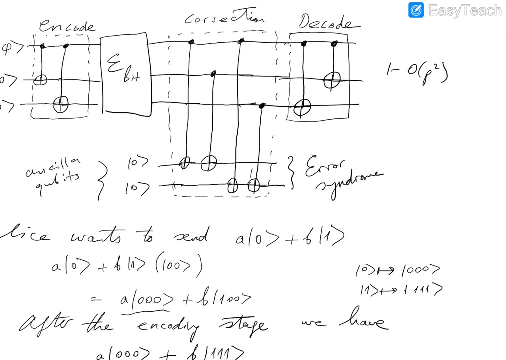 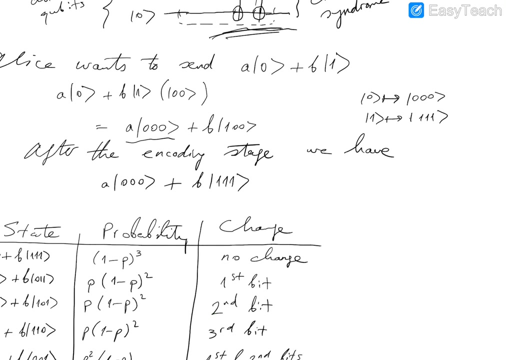 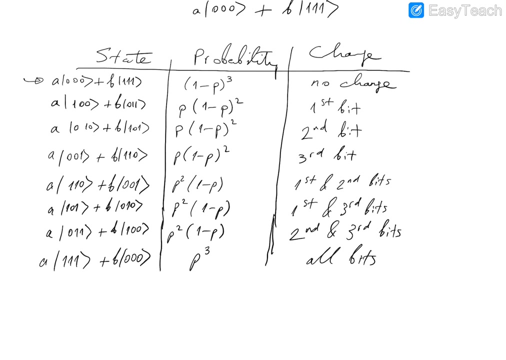 And Bob's going to use these qubits to gather information about the error. And after applying the CNOT gate, the compound five qubit state. So there are five qubits in total in the system. So after applying the CNOT operation here, 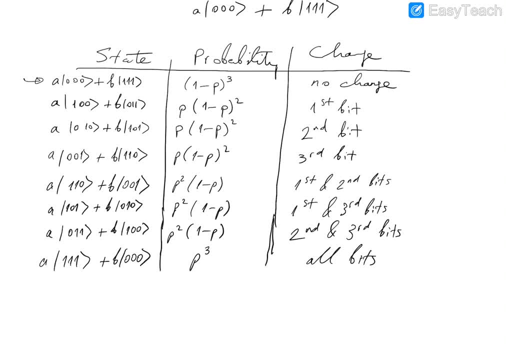 I'm going to modify this table, So in this case the last two qubits will be zero- zero. In this case we have one one, Here we have one zero, And here we have ket- zero one. This is zero one. 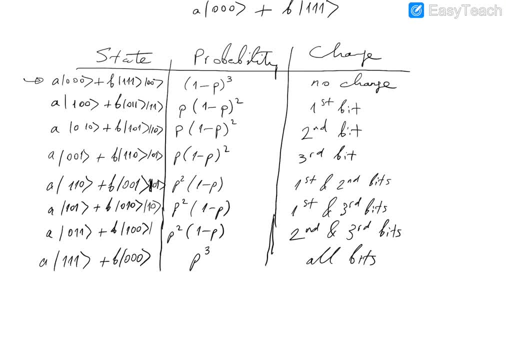 And here we have one, zero, One, one. And look, And lastly, we have zero, zero, OK. so so next, Bob measures the two and Scylla qubits in the canonical basis, OK, and essentially what we get is basically two classical bits of information. 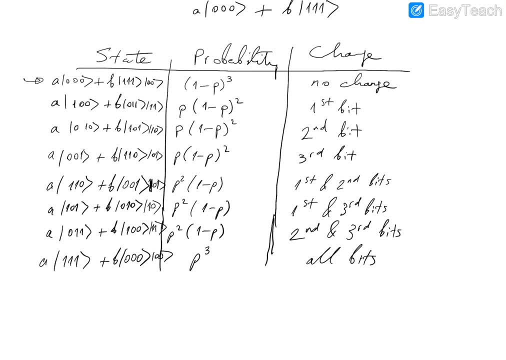 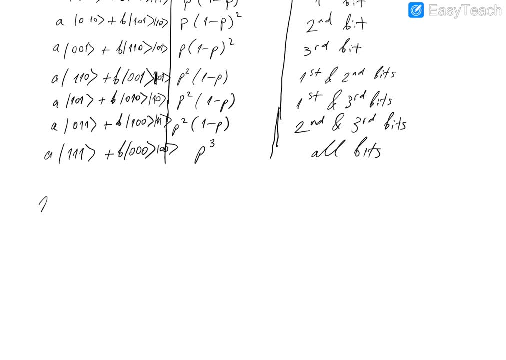 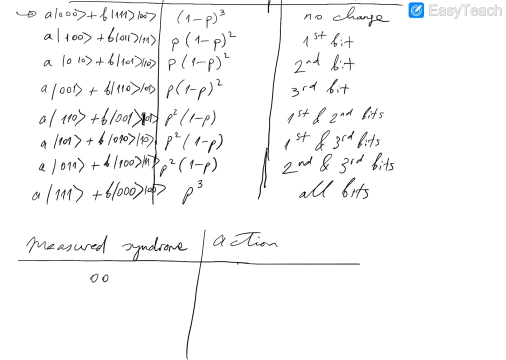 So this is what we call the error syndrome. It's the information about the error. Now, if Bob measures Measured syndrome On one side, and the action that Bob takes, If Bob measures zero zero, Then Bob does nothing. I'm going to explain why. 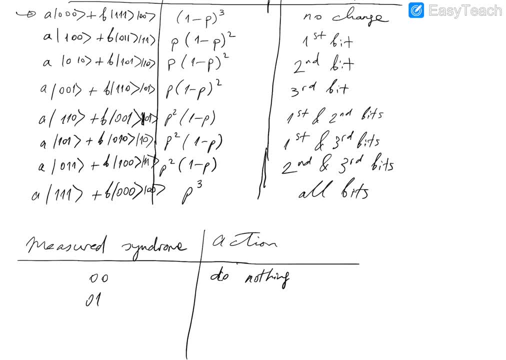 But if Bob measures zero one, Then He just flips the third qubit. Flip The third Cubit. If Bob measures one zero In the error syndrome, Then he flips the second qubit. And If he measures one one, 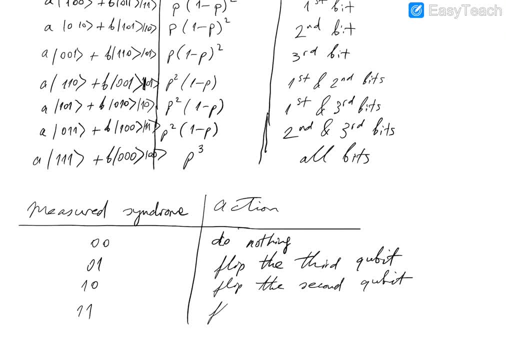 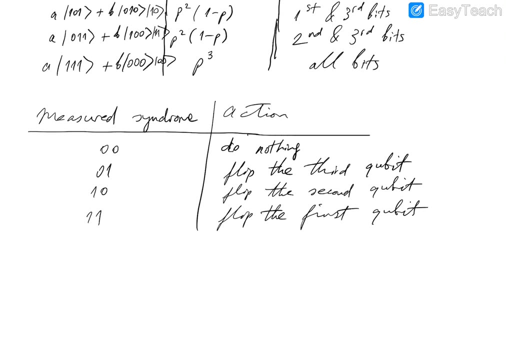 Then he flips the first qubit. So OK, Let's Let's suppose, For example, that Bob measures one zero. OK, so suppose Bob measures one zero in the error syndrome. OK, Now let's examine the table about. 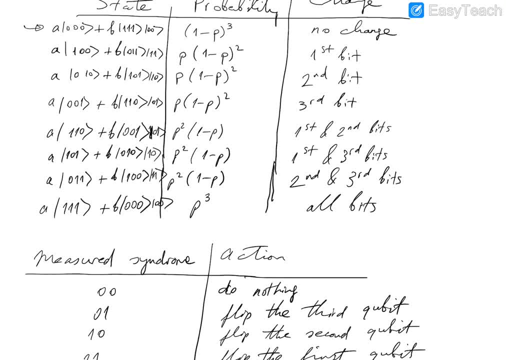 If he, if he, measures The error syndromes as one zero, Then He must have even received This state Or that state. In fact, there are the complements of each other. So we have a zero one zero, And here we have a one zero one. 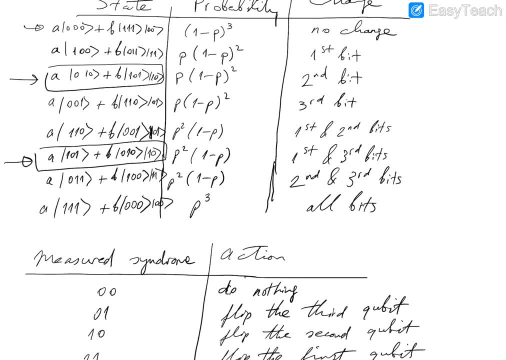 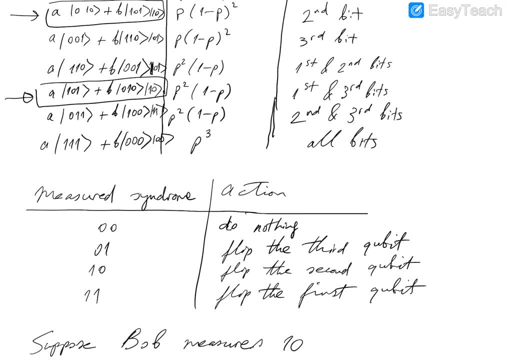 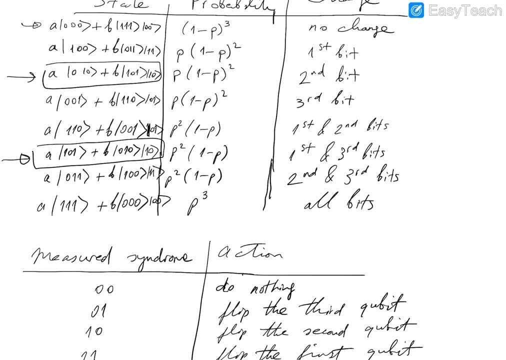 Here we have B one, zero one, And on the downside we have B zero one, zero. OK. so, But which one is more likely, We can ask? Well, Certainly, this one Is more likely to happen. It's more likely that. 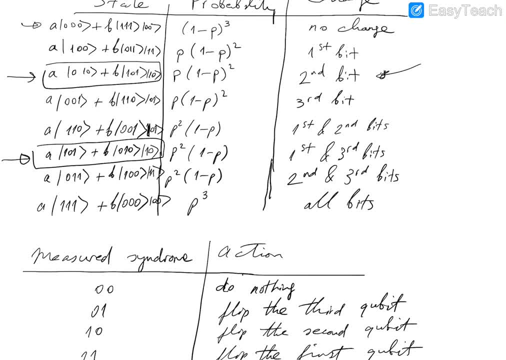 That only one qubit gets corrupted, Rather than two qubits get corrupted, Right? so The probability of this State Bob receiving this state, Is P times one minus P squared, But the other probability Having this state Is P squared times one minus P. 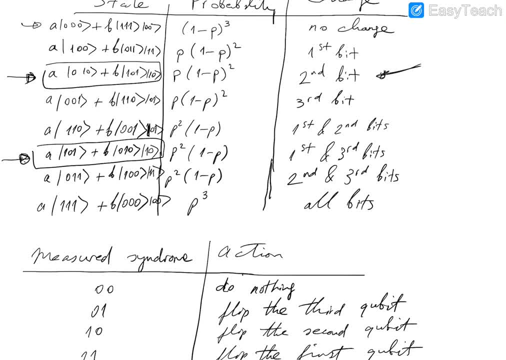 So it's more likely that Bob has This state instead. So Then, what should Bob do? Well, Bob corrects the state by applying The not transformation on the second qubit. then, Since the second qubit Was changed during the transmission, 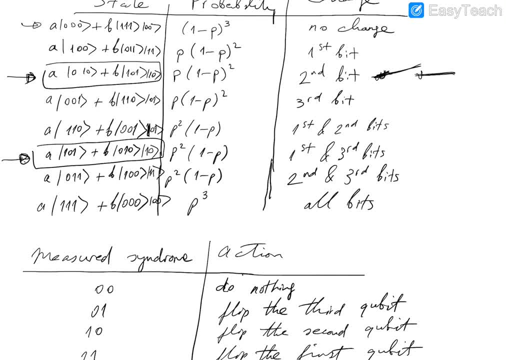 Then Bob is going to apply And since this state is more likely to To be received In the receiving end, Then Bob, It's It's more reasonable to apply This Correction, Applying a, not transformation. on the second qubit. 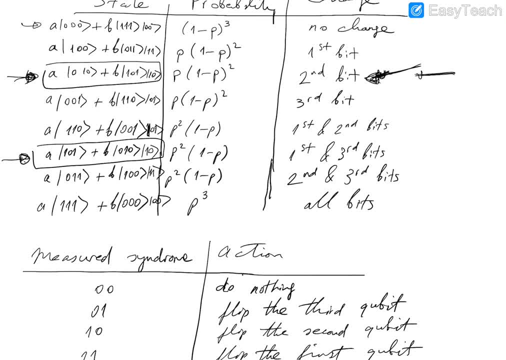 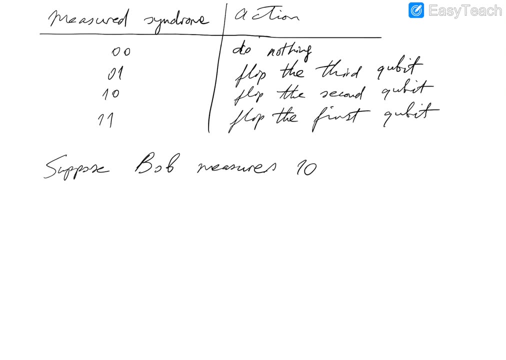 Rather than applying the transformation With a not transformation on the first and third qubits. All right, so, So Let's. But this doesn't quite give Alice's original states, You might ask. well, Alice wanted to send, She wanted to send. 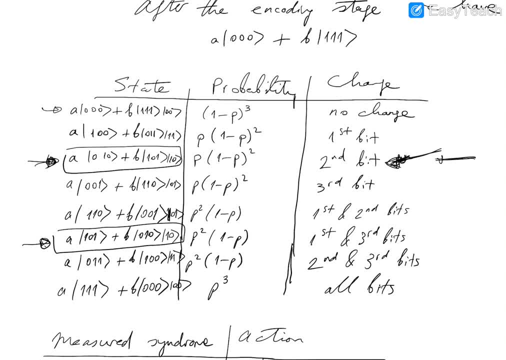 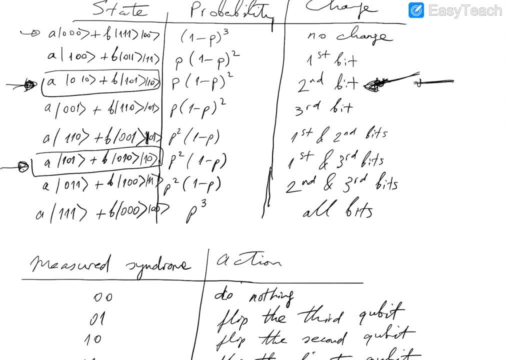 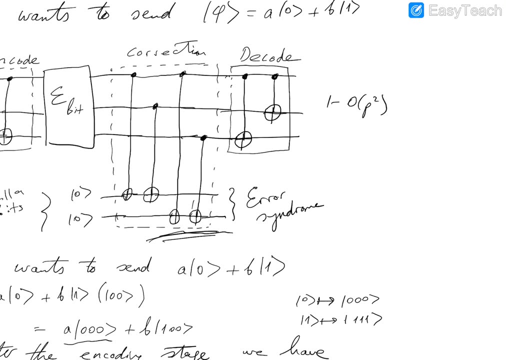 A zero plus B one. So how are we going to get that? Well, Bob applies See not transformation. on the third and second qubits, If we look at the diagram here, Here Taking the first qubit as As As the control qubit, 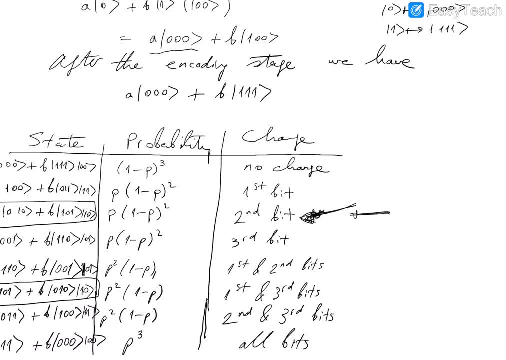 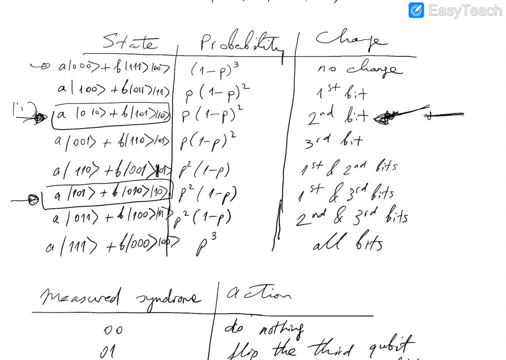 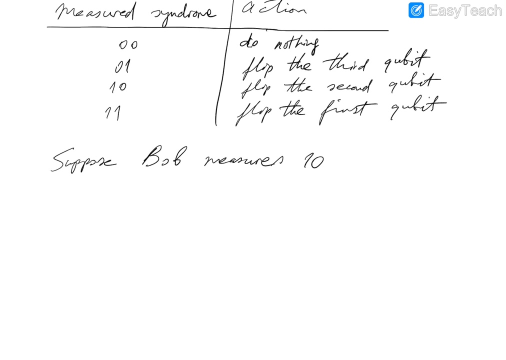 So Assume that Bob either receives- Let me call these, I Maybe star And dagger, Okay, So he either receives a star state or the dagger state And if he applies The decoding operation, The final state that Bob receives- 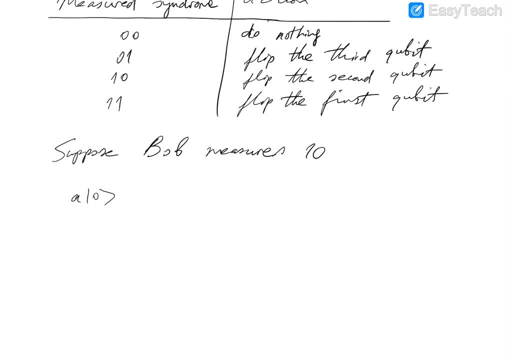 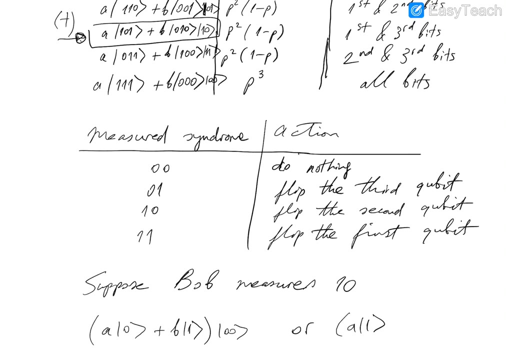 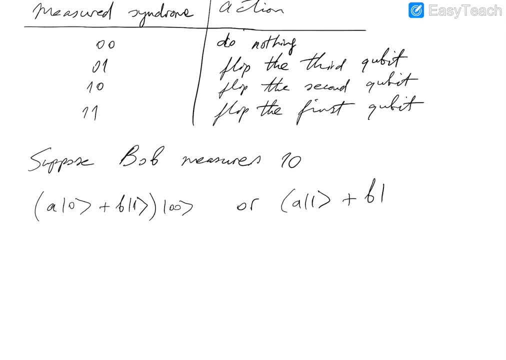 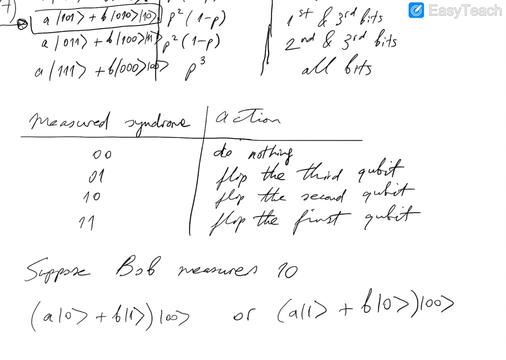 Either going to be A zero Plus B, one Zero zero, Or it's going to be. If he receives a dagger After applying the decoding operation, He will get A one Plus B Zero Zero zero. The last two qubits are: 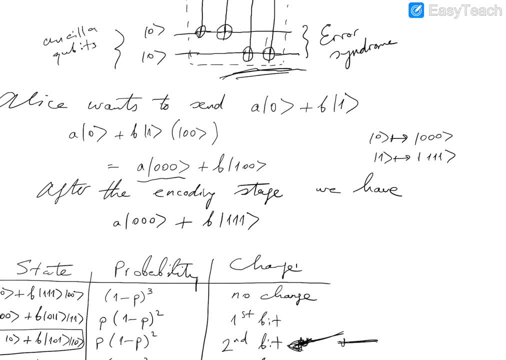 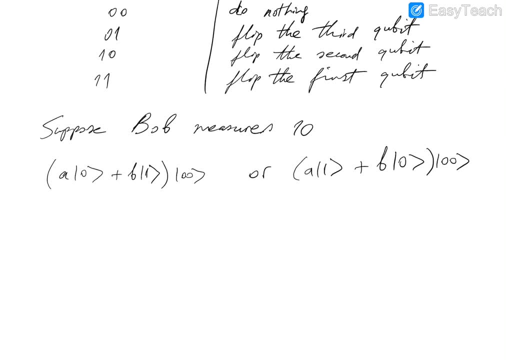 The qubits from The encoded states. Okay, All right. so Now, at this point Bob doesn't know Which state he has, But the important point is that This method Has a success probability greater than One minus P The failure probability. 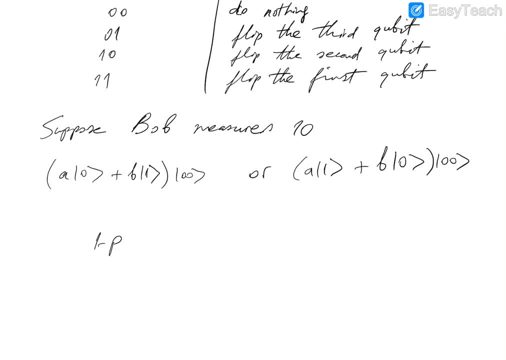 That at least two qubits are corrupted By the faulty channel Is less than P, So the probability that Bob Fails to obtain Alice's original state Is Is bounded by P squared, Whereas it would have been, So this is with error correction. 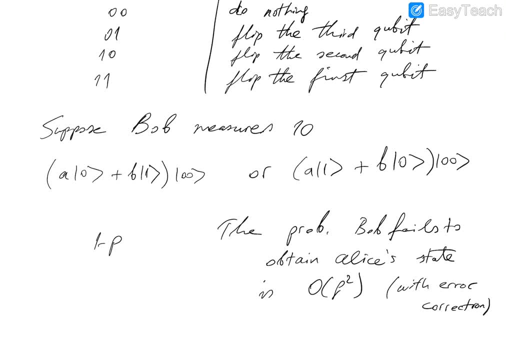 With error correction, Whereas it would have been Bounded by P If no error correction Had been used Without error Correction. So, of course, with more qubits, We apply the same idea here And we get More. We get better. noise suppression. 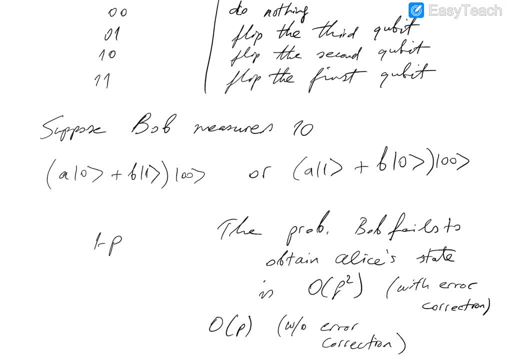 And the success probability Will increase exponentially. Okay, So this is how The bit flip model works, But this is not Really exclusive to quantum Computation. What's more exclusive to quantum Computing Is the phase flip error: Phase flip error. 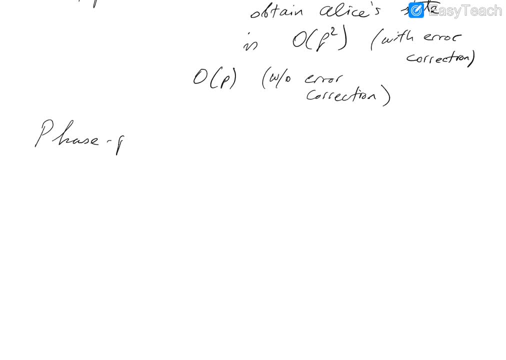 So If we are given something like A zero Plus B One, This gets mapped to A Zero Minus The Phase Flip Error. So If we are given something like A zero Plus, 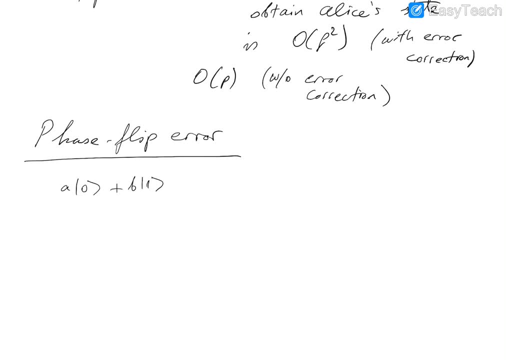 B One, This gets mapped to A Zero Minus The Phase Flip Error Plus B One. Or, similarly, If we have A Zero Minus B One, This gets mapped to: 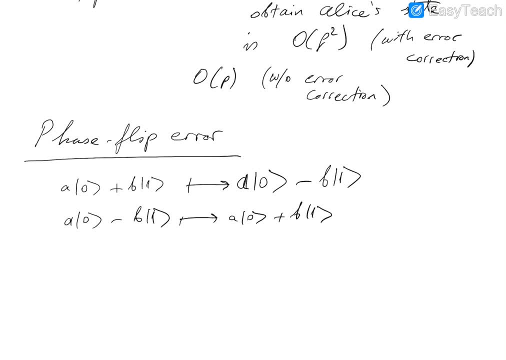 A Zero Plus B One, So it changes the relative phase, The sign Of the Of the Quantum states. So This kind of error, The phase flip error, Is not found in Any classical Error correction. 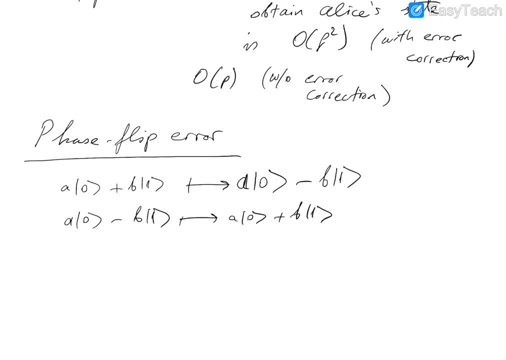 Because There is no Corresponding Phenomena For The phase value In classical computing Right, Because The Concept Of The phase Is unique To quantum computing And Though This is a restricted form, 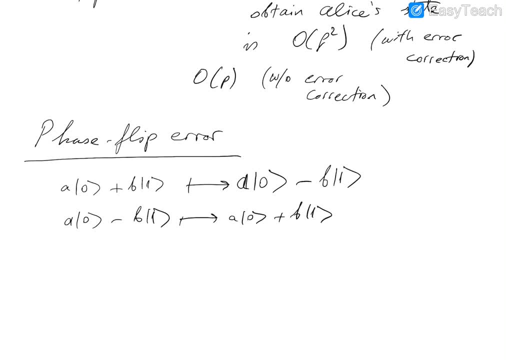 In fact We will see Later on What That We could Have Phase Defined By Generally By This Number In the Exponential Form, Right? So If Phase Flip, 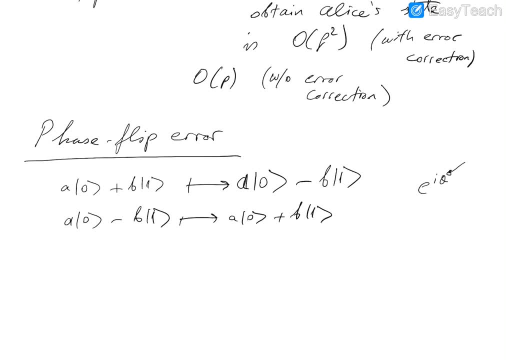 Error. In fact It Changes This Phase Value, Theta, Which Is A Real Number. So That's Why We Have Continued Many To Correct The Phase Flip. 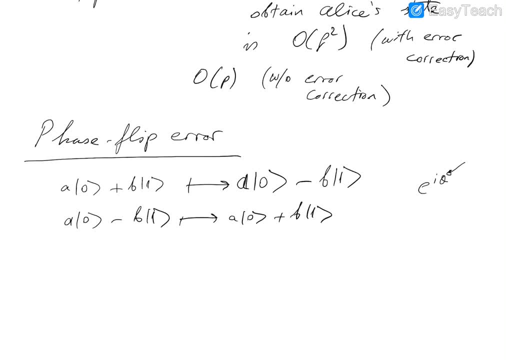 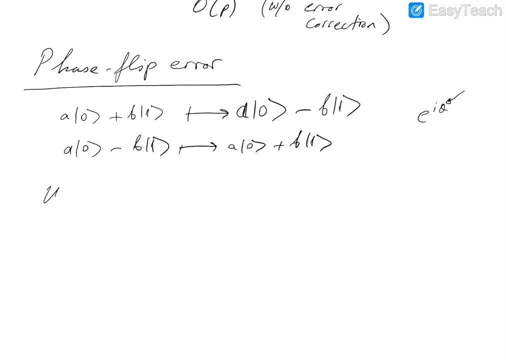 Error, And One Way To Do This Is To Transform The Phase Flip Channel Into A Bit Flip Channel, And We Do This By We Turn. 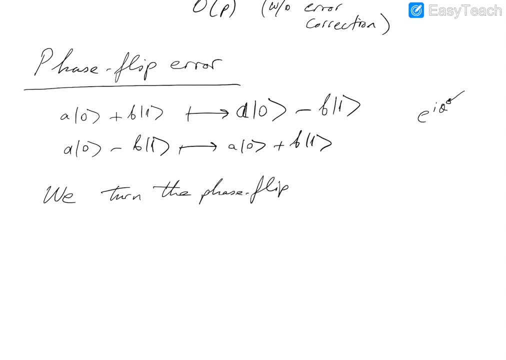 The Phase Flip Channel To A Bit Flip Channel Using Change Of Basis. Okay, So Suppose That This Turn On A In The Phase Of Challenge. 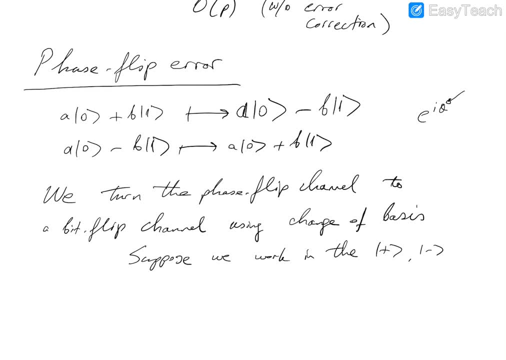 At. So At The Basis It Takes A And To To To Change The Phase Of Change And To minus 1 over square root 2, 1.. Okay so. 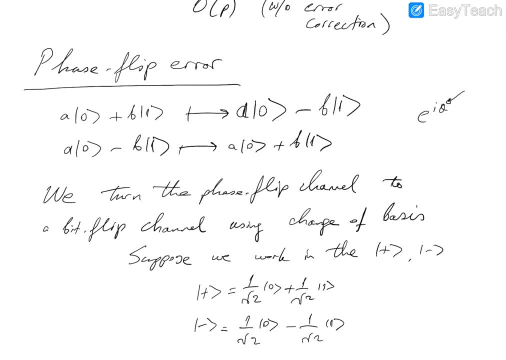 the idea is the same, except that now we work under the sine basis. So the basis change is performed by an application of the Hadamard transform, because Hadamard transformation is simply used to change the basis from the sine basis to the canonical basis. 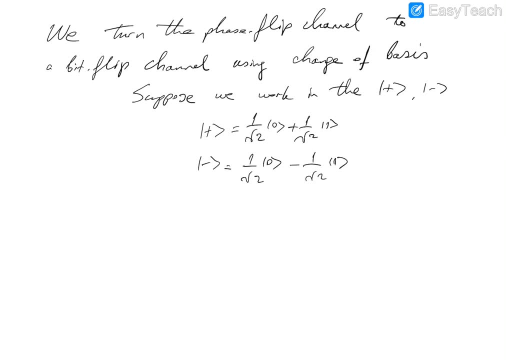 So we use the Hadamard transformation and it's inversed at appropriate points in the procedure to perform the basis change and we still use the bit flip error model. So I'm going to give you the circuit diagram for this, for the phase flip code. 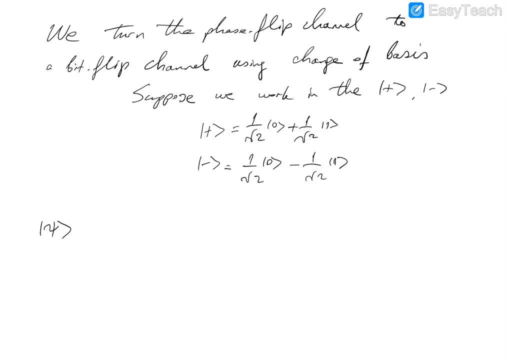 So we start with psi, the state that we want to transmit. We have two ancilla qubits set to 0. So we take the first qubit as the control qubit and then apply a CNOT transformation on the second qubit and then